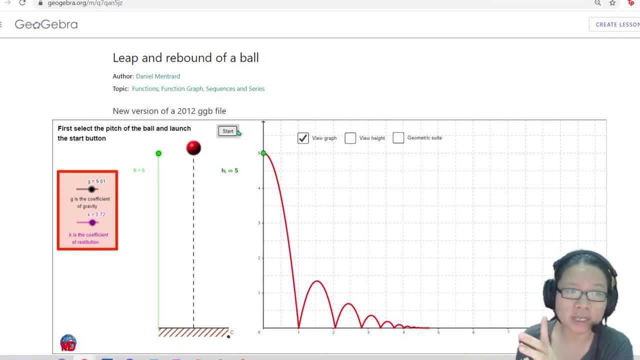 involving a rebound, or basically the collision of the ball and when it comes up again. Okay, so you may be wondering: is there a case where there is totally no loss in energy, Where my height is always the same, like this one? Well, in the ideal case, yes, But this is an ideal. 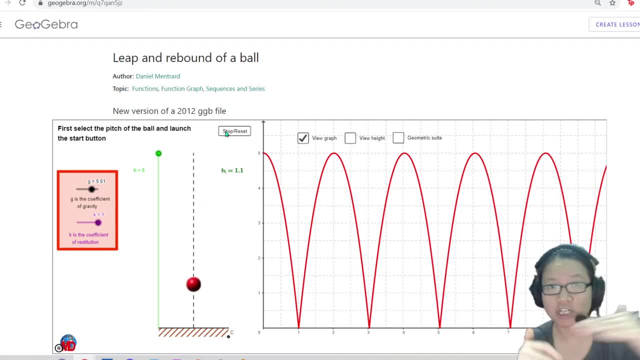 case. So we will do the ideal case where there is no loss in kinetic energy. So we will do the ideal case where there is no change in height and then followed quickly by increasing the rate of loss of kinetic energy. Okay, so every time you rebound, you don't get back to the same height. 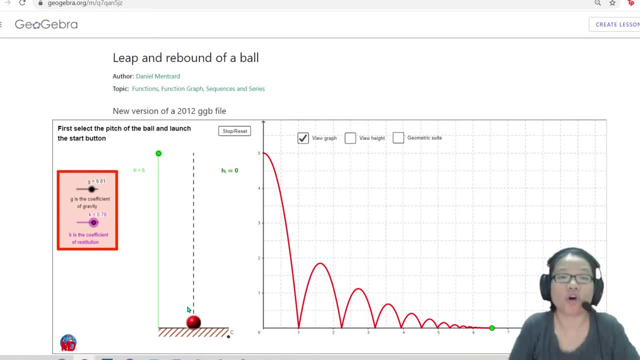 Of course, the material of the ball and the type of floor will get to influence how much the kinetic energy is conserved. So let's put all of this into a graph. First, to help us visualize this, I am going to just roughly sketch out the scenario. Okay, so let us set our parameters. 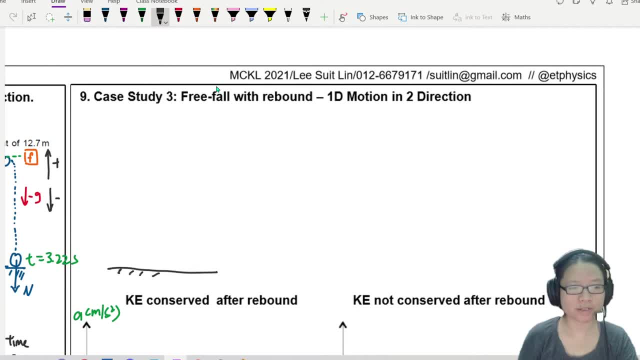 first have the ground somewhere like this: okay, and i will drop a ball from a certain distance. okay, let's say here t is equal to zero and the ball is at a height h above the ground, or rather, since this is the initial height, i will call this h naught zero for initial okay here at. 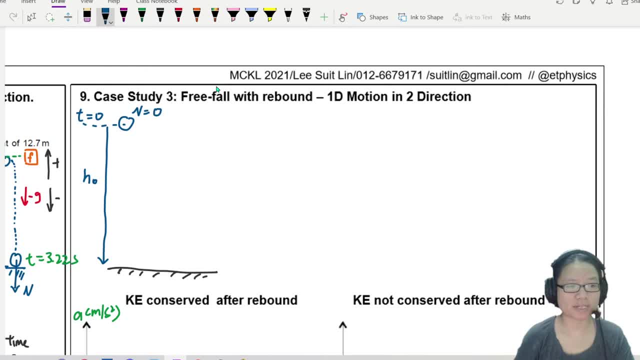 this point the ball's velocity is zero. it will accelerate, accelerate, accelerate until it hits the ground. okay, so let's say it hits the ground here and when it hits the ground the ball will have a velocity of v1. and to make our life easier on this friday night, i'm going to just give v1 a. 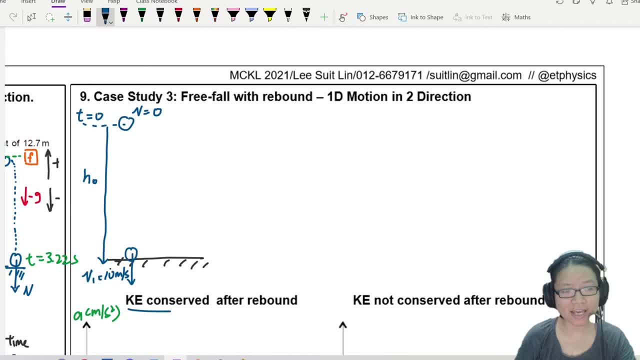 value, let's say 10 meter per second. so if ke is conserved, this means that the ball will leave the floor. okay, along, they are along the same line. i draw them side by side so you can see. but actually they are the same line, all right. 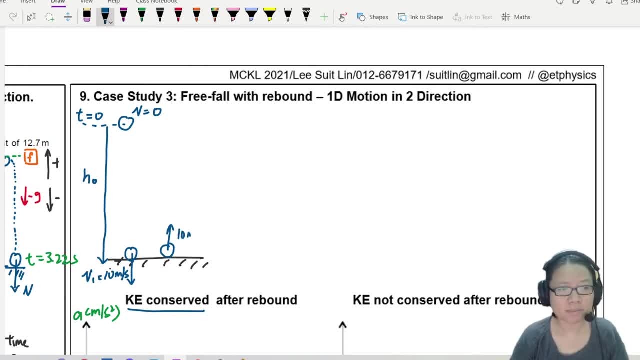 so this one is also going to leave at 10 meter per second. this is also a magnitude of v1, but since we all know that velocity is a vector, so we need to assign a sign, positive or negative. so you have to decide. i think i'll just follow the normal convention. i'm going to draw here so that 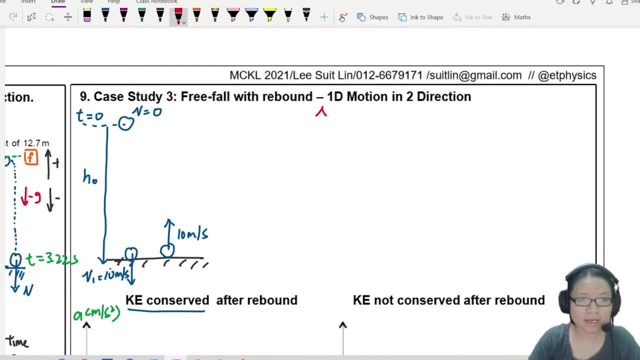 we can see very clearly. i will take the up direction as positive and the down right direction. okay, so this would be negative 10 and this will be positive 10.. and since there is no loss in kinetic energy, ke is conserved, then this ball can return to its original height, h1. okay, so what? 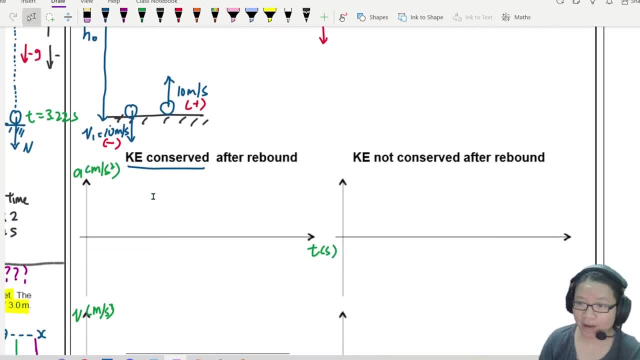 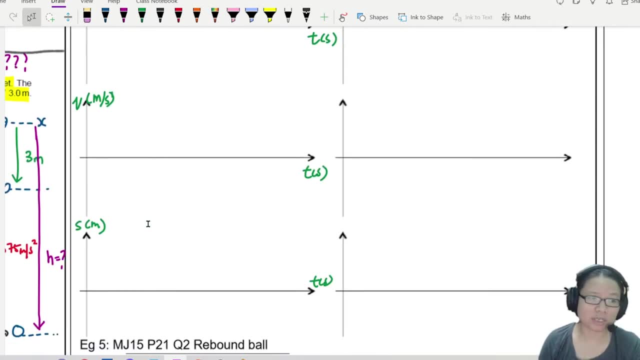 graph are we going to draw? we will draw the acceleration graph, the velocity graph and the displacement graph. okay, so the easiest one to draw is actually: i mean, i don't know, you can start anywhere, so let's say i start with velocity. okay, so for the velocity graph, right, um, we start. we. 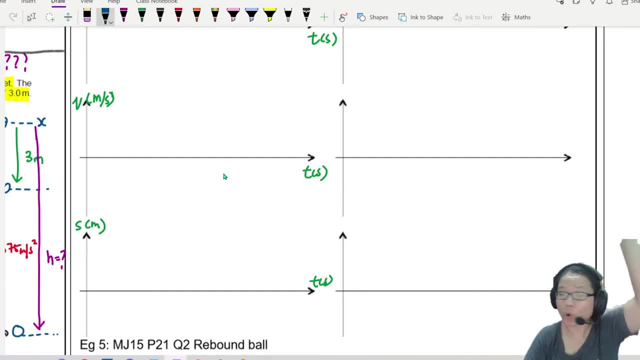 let we you imagine: or you hold the ball and then you let go, so the ball starts with zero and then it will accelerate downwards. so i'm going to just give it a negative value of b until it hits the ground. so this value here, when it hits the ground, is negative 10. okay, then after that, after it hits, 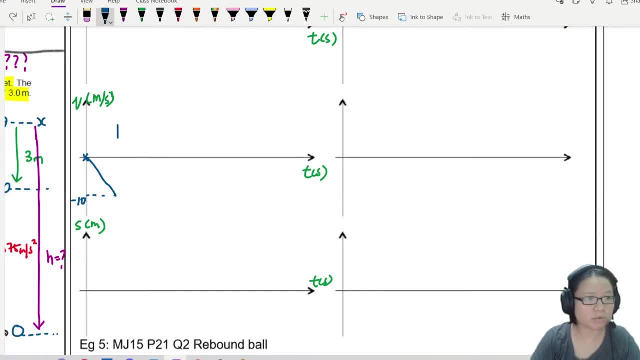 the ground. it will rebound. okay, probably rebound somewhere here, like this. and then this one here is positive 10. okay, so it goes back, leaves the floor. so i'm going to label some points here. so you know, this point here is impact the ground, and then this point here we will leave the ground. 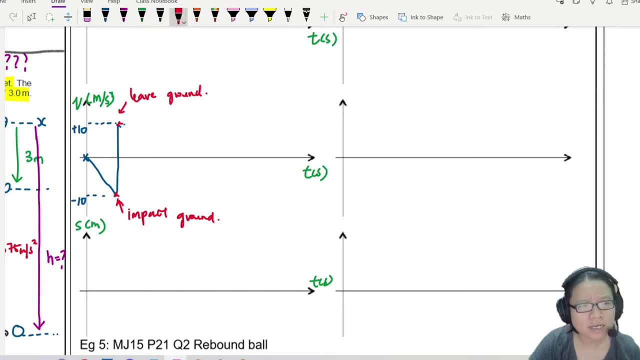 you may be wondering, miss the, the contact time? uh, very short, is it? yes, very short. so when we draw at this scale cannot really tell. or even if you can tell, it is a little bit tilted when the rebound time is significant. think about the trampoline question. 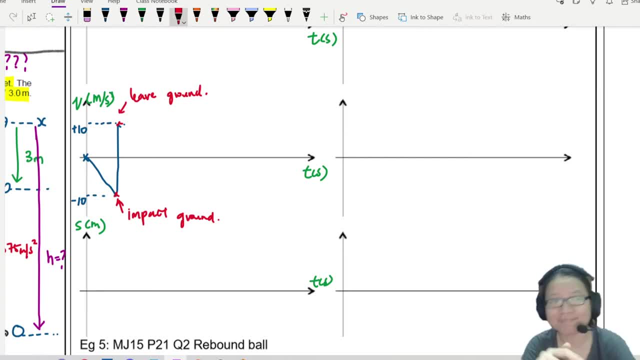 that you have done okay. so there's a partial question that involves trampoline. trampoline questions will have a longer rebound time, but in this case i assume the floor is solid, as solid as your interest and ability in physics. so rebound time very small. so right now it will travel it. 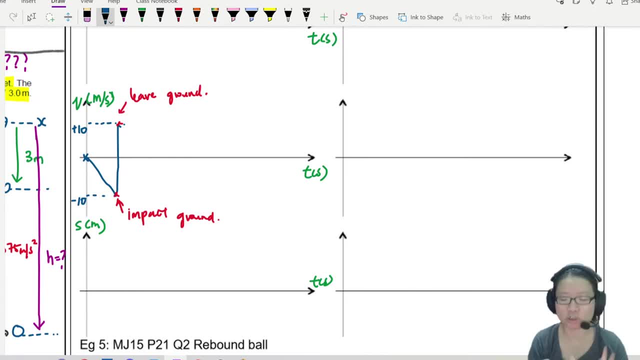 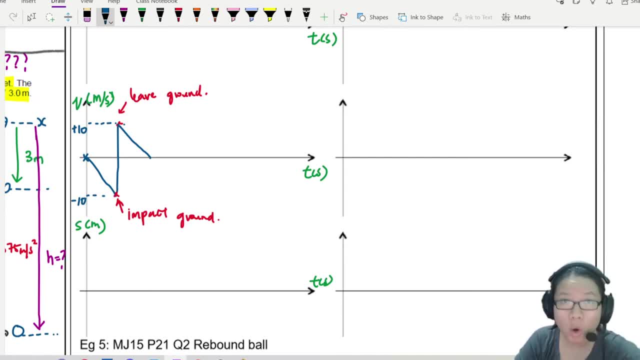 stay here, right? what's it going to do? it's going to come down, so it will increase its speed in the negative direction. okay, so here it leaves the ground, it will slow down, it will slow down, it will and stop here, and then after that it will accelerate and move faster. and faster means. 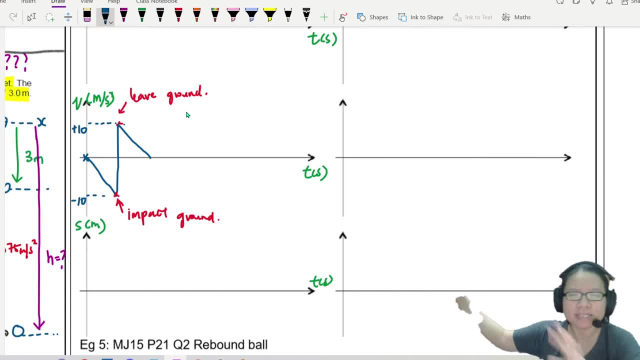 this is like the graph that we draw, just many, many times the graph as that we draw, correct, it's putting all the graphs together, okay, so this one will look something like this and, of course, it's going to reach the same- uh, same- height. so let me try to draw the line a bit better. 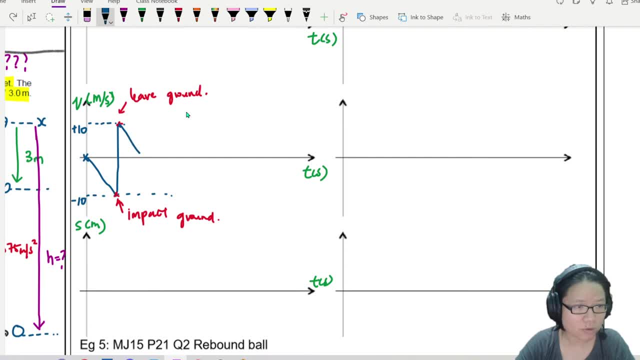 these two lines are obviously parallel, okay, and the reason why they are parallel is because they will have the same, uh, acceleration. we'll talk about that later. so maybe i will draw it for another rebound and then i'll call it a day okay, so something like this, and continue so on, so forth. 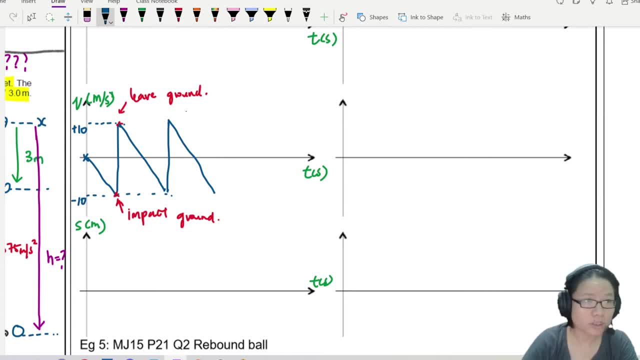 right. so in this case, right, do you know what is going to happen? what will happen here is, you will have a scenario where the area is the same. this value of h, this area here, is the same as the other area here up here. they have the same area, in fact, the area of all these graphs. 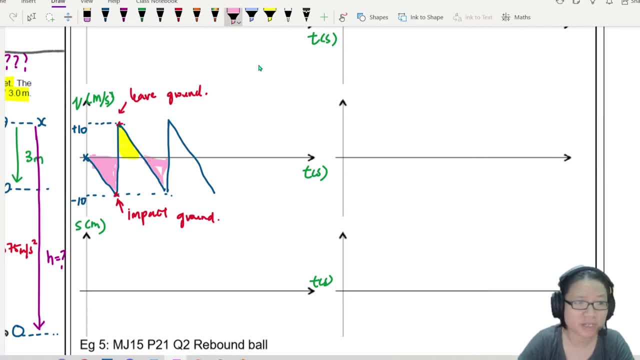 are the same because why? the area represents the rebound height. okay, so this will be h not. this is h not, this is h not. in fact, everybody is h not. okay. so you might be thinking: why are miss? why is it that the area is there a dz, i guess, so it doesn't have? in fact, it has a dark yellow one. 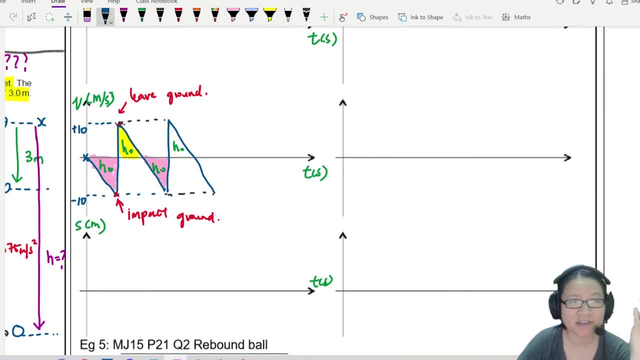 is positive and negative, though we get positive and negative area. let me finish this one. this is also h naught, because sometimes the ball is moving down, sometimes the ball is moving up- okay, so it depends on whether it's moving down or moving up. so if it goes down, hits the ground. 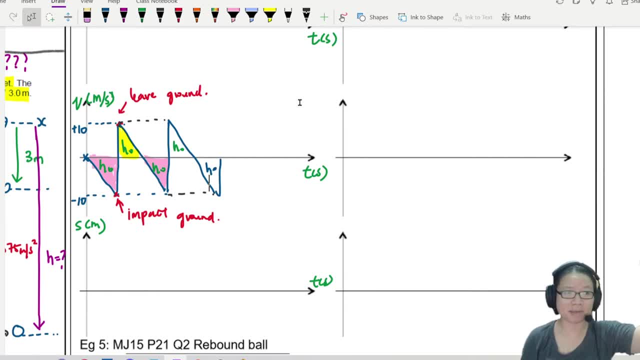 leave and go back to the original point. here this is at maximum height. so this, where it touches the axis, here and here, these are all at maximum height. you return back because you drop from here, hit the floor, come back up, you return back. this is the maximum height. okay, so these are examples. 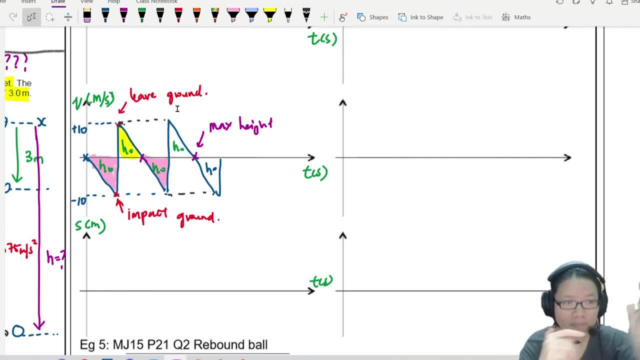 of the vt graph: okay, the peak is the same and these lines are all parallel. okay, let's talk about the parallel lines now. parallel lines here: okay. so if you look at the gradient here, okay, let me label this colors to use. so, all this vt graph, the lines are parallel. this line and this line is parallel. 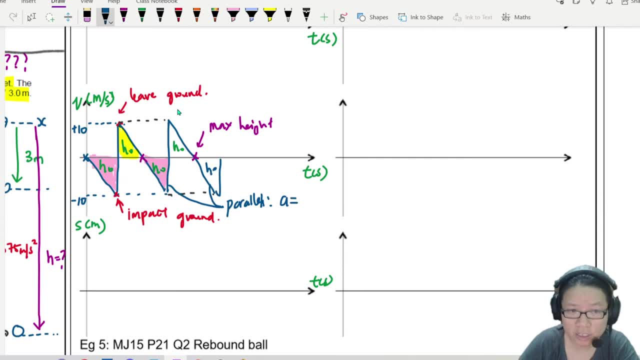 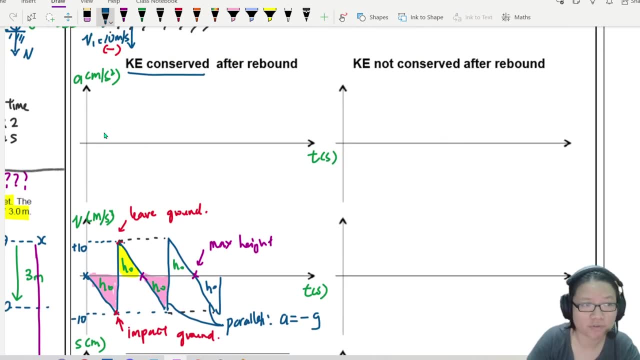 okay, and they are parallel. to show that the acceleration is equal to negative g. okay, so if now i want to draw the acceleration graph, it is relatively straightforward. you will expect a negative g, but, teacher, you see, ah, this part a bit strange. this is weird sharp edge here like a bit weird, right? ah, yes, so the acceleration is gravity, unless the ball. 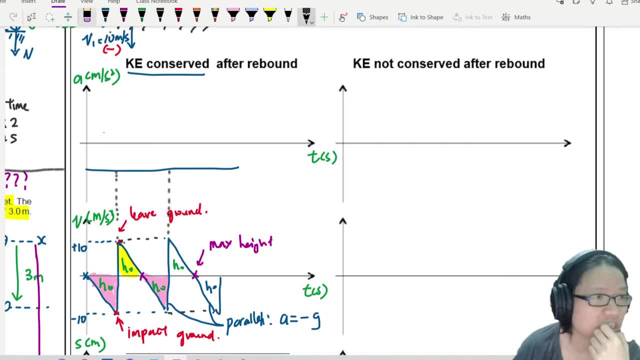 is whack the floor. okay, so that means i need to adjust a bit. ah, you also adjust with me. okay, draw these graphs with me. all right, don't just watch me draw. so for a period of time there's a spike. this is the impact force. okay, this is when the ball is in contact with the ground, because time is very 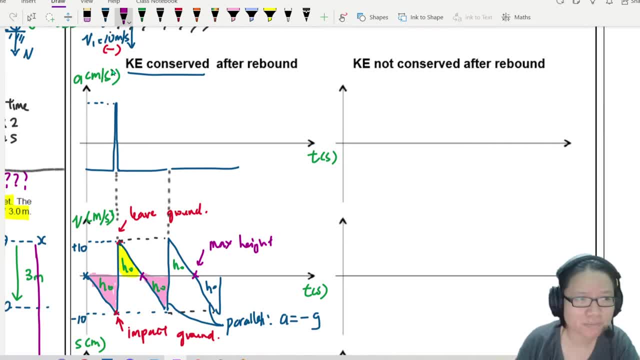 short, so the force is very big. that's why the ball can change direction. so this one is all during impact, okay, during impact, so, and because everything remains the same. so basically this scenario will repeat, repeat, repeat with the same values. otherwise this one is negative g, okay. 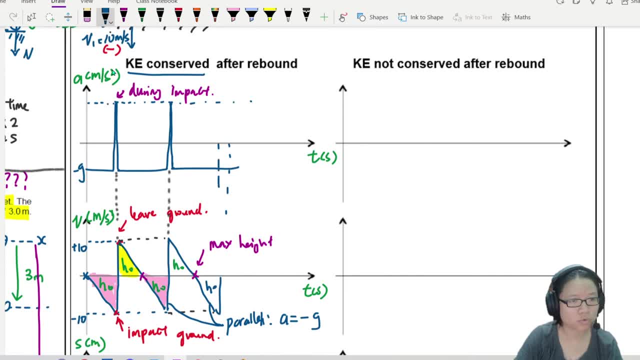 so, if you want to, i can draw the next one for you. this one here will also be something like this thing, thing, thing thing, do la like that la. okay, all right, great. you also notice that if i draw this properly, this time and this time is the same. so this gap here, this t. 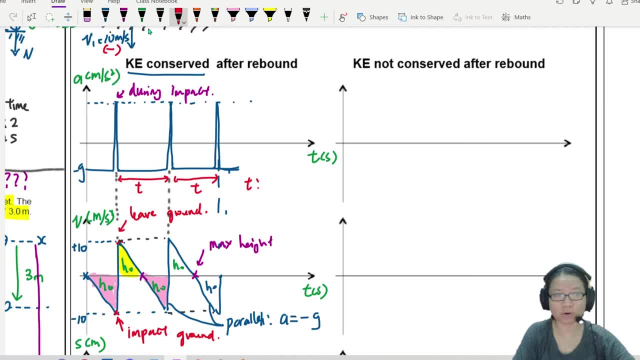 t is the time between the ball hitting the ground, go up, come back down and hit the ground again, so this is called time of flight of the ball. all right, okay, draw v, draw a, because we look at the gradient, which is easy to look, because this one very steep, very positive, so it's a large positive number. okay, what about the? 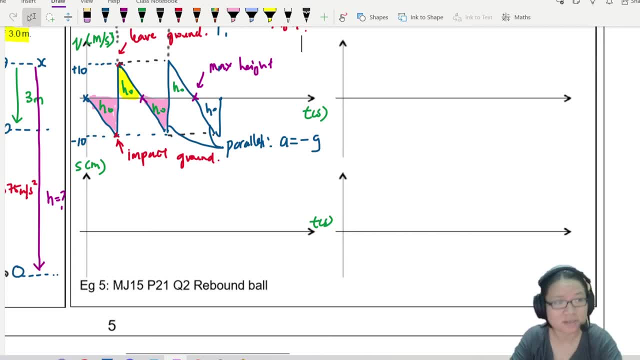 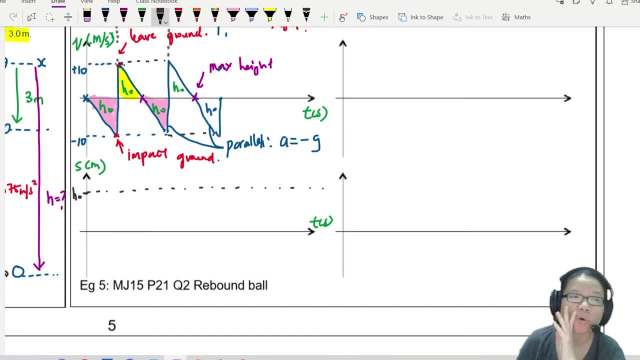 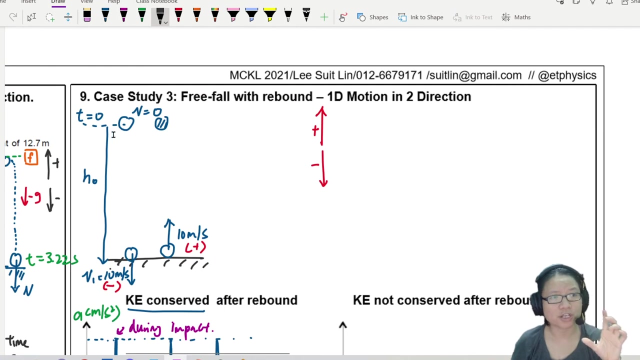 going to be h naught, okay, so i now need to figure out when is it that we reach maximum height? okay, so we started off at maximum height and then we let go of the ball. okay, and then here is where the ball touches the ground. so i'm going to treat. okay, let me see. did i label correctly? i will treat the release position. 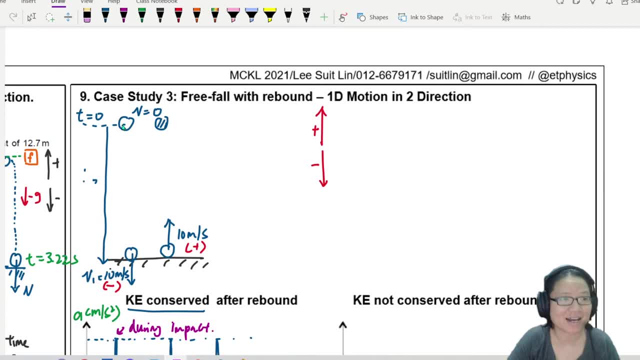 as h naught, i measure from the ground. okay, so because i want to replicate the graph that i see just now means you measure from the ground and you measure from the top. the graph is different. yes, the graph is different. try and draw and see what happens if i measure from the top, but in order to get the same one that i got from. 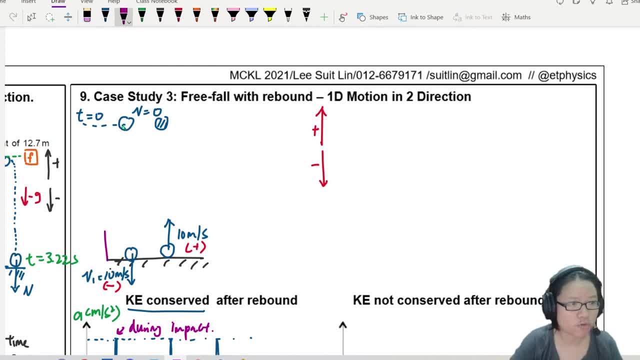 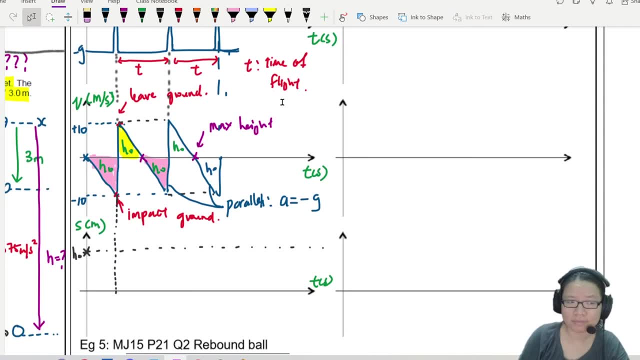 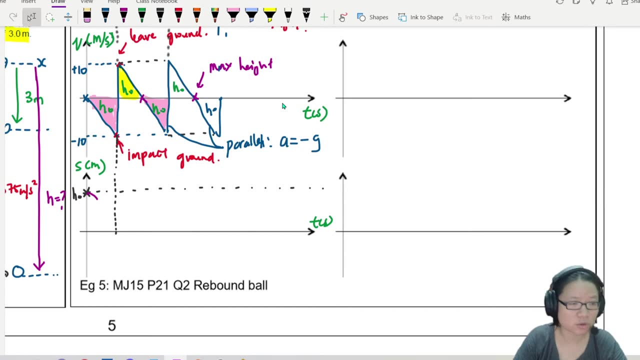 the simulation, i must measure h from the ground up, so i will start with h naught. okay, i will assign it as homework, all right. so anyway, this one here. you will start at h naught, it will go down and then this is where it touches the ground, so it will accelerate, accelerate, accelerate, accelerate. 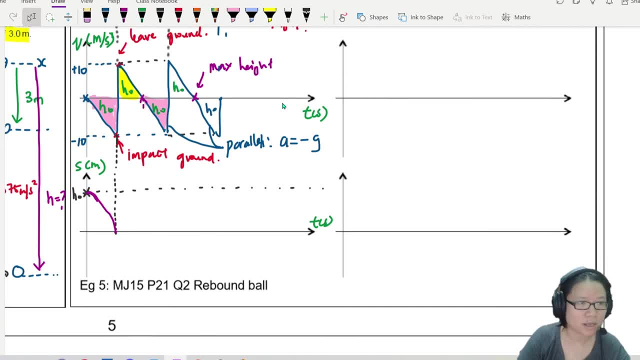 steeper and steeper and steeper, and here is where it will have maximum height, so it will go back up boing. so all this part here of the graph, if you draw it or you graph it carefully, they are all identical: boing, boing and this will keep boing, boing in or rebounding. 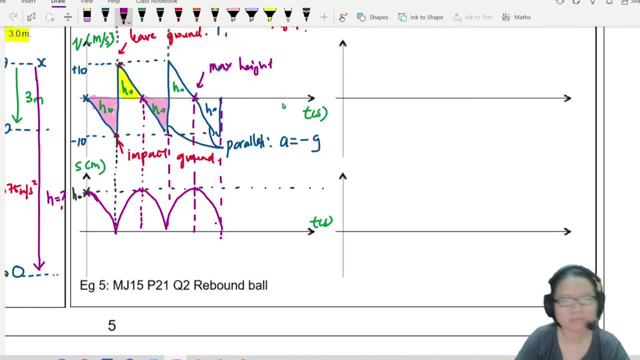 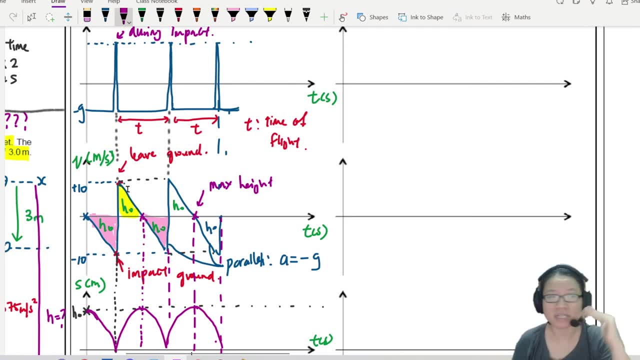 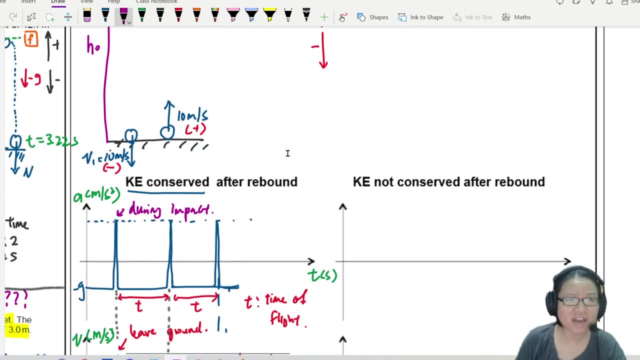 rebound, rebounding until forever. okay, this is ideal scenario. maintain the same speed- 10 at every single rebound. maintain the same height- h naught- at every single rebound. but you know life is not perfect. miss, you know, we lose energy. i attend, i boing, boing from maths. 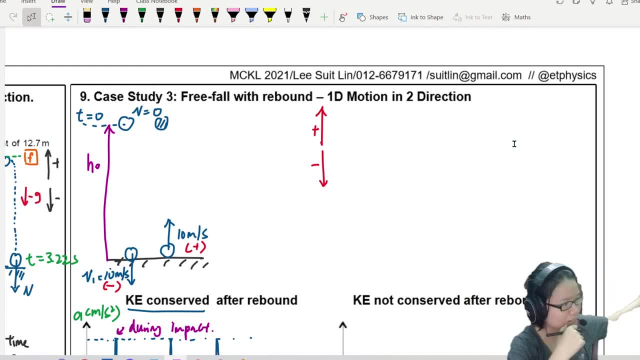 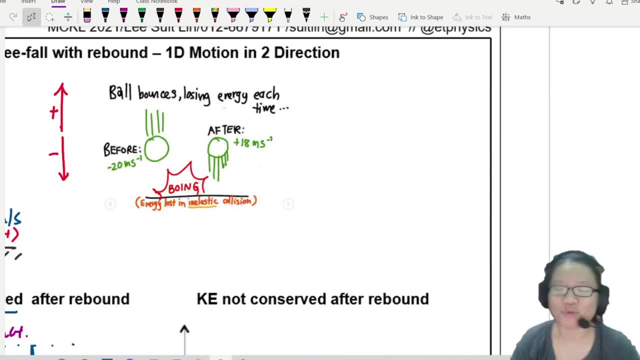 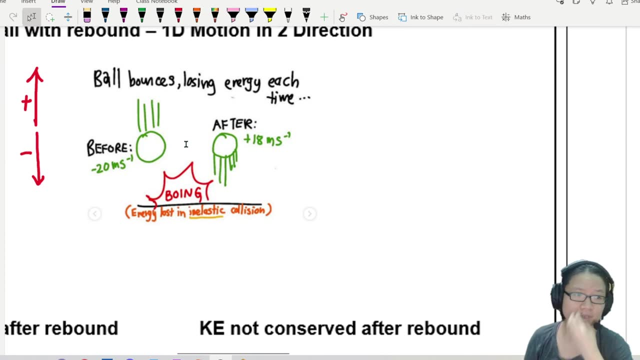 boing to chemistry, boing to bio, boing to computer science, boing to physics. my energy is gone. so don't worry, i got you. i will draw that graph now. here's a scenario where the kinetic energy is not conserved. okay, so let's say, every time the ball bounces, it loses energy, so it goes here, boing goes up. 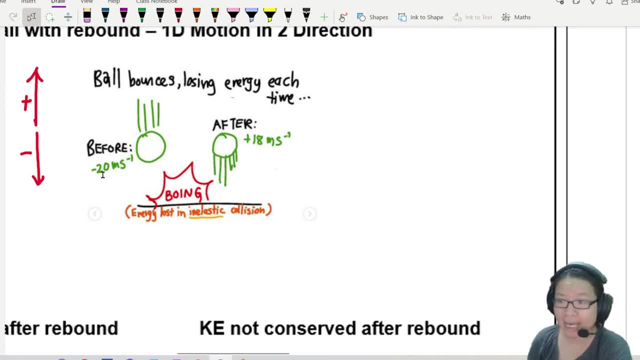 lose energy from negative 20 to positive 18 meter per second. we call this collision in elastic, so take note of the term in elastic, because we will come back and we'll see this again or maybe you'll do some question and you encounter: in elastic this means ke naught. 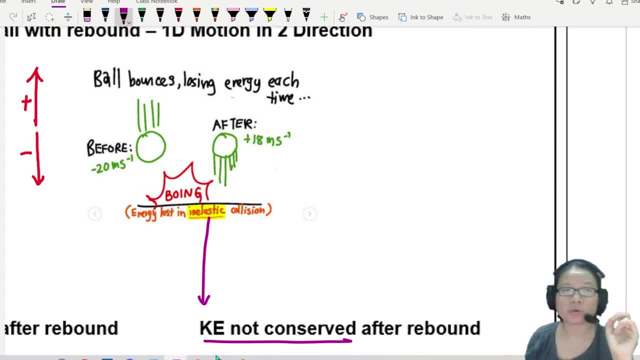 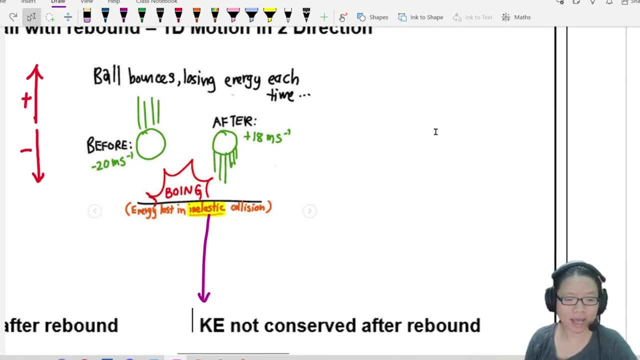 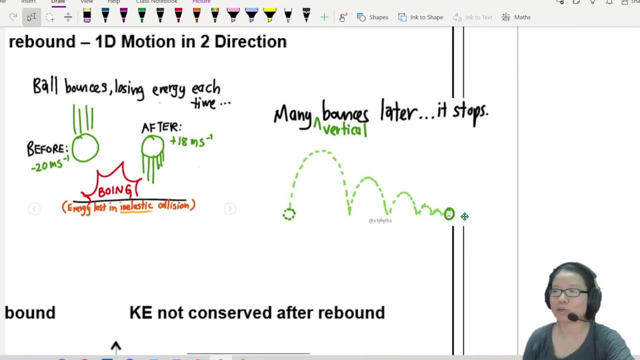 is a okay. so it will leave at a smaller speed, means it will rebound at a smaller height and you will tend to get a graph looking like this: many rebounds later. it will stop, teacher. this one looks like the st graph, correct, all right, so let us graph the acceleration, the velocity. 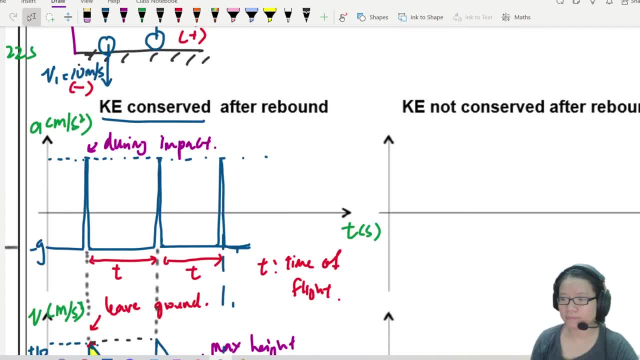 the displacement. okay, so let's start by modifying the graph that we already have. this is acceleration time, but every time we rebound we get the same amount of force because the ball will collide with at the floor with the same speed. but if, let's say, your ke is not conserved, then you will get a graph that looks a bit where the peak will decrease. 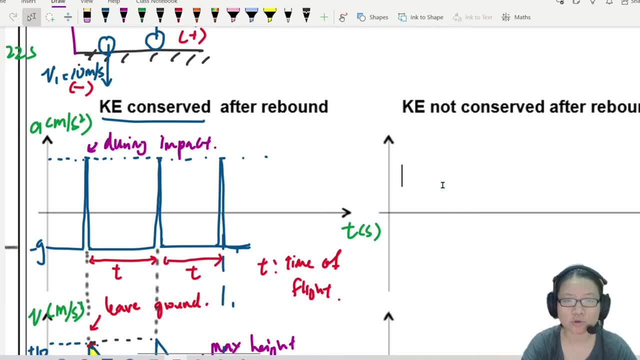 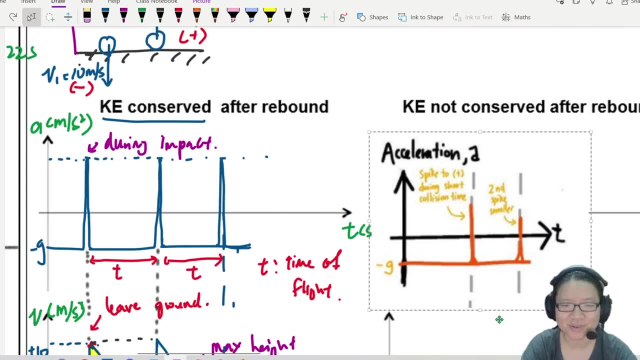 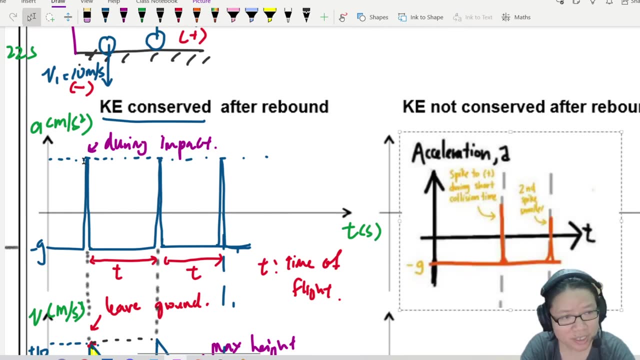 decrease, decrease, right. so it's going to look something like this: oops, too many. okay, it's gonna look something like this: all right, so right now you can see your that i draw, or whether we have a graph for this one. you will see that this peak. 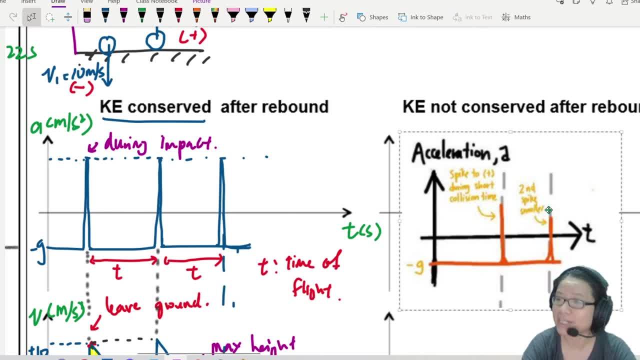 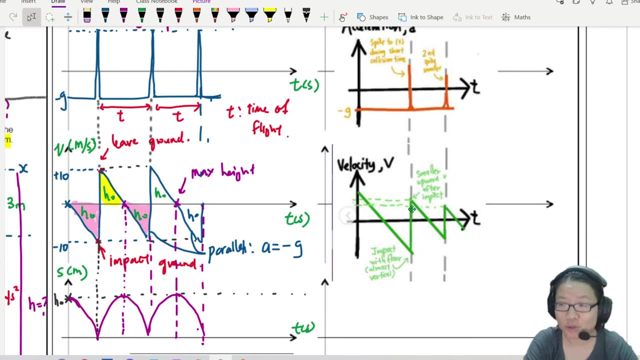 will decrease. okay, smaller and smaller each time, so eventually it will decrease to zero. all right, so acceleration. okay, let us now modify velocity. how would this velocity graph look like? so, if you look at this new velocity time graph, obviously we won't be able to return to the original height. okay, and you will see that every time there's. 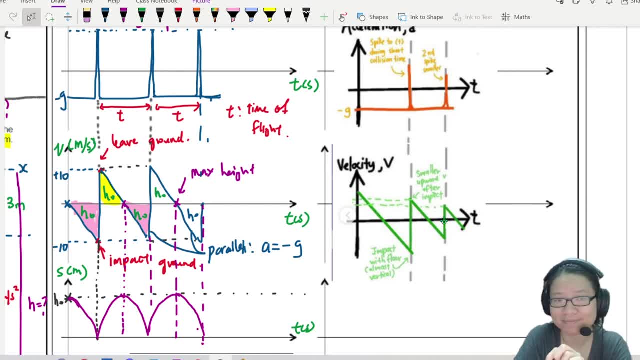 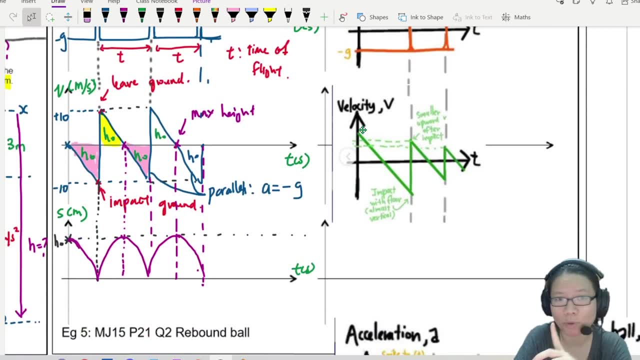 impact. the peak gets smaller and smaller and smaller. all right, so this graph is not specifically for this motion. okay, if you check out the graph, it starts with positive v. so basically, the sign convention is different. you think about how the sign convention will look like, but what we're? 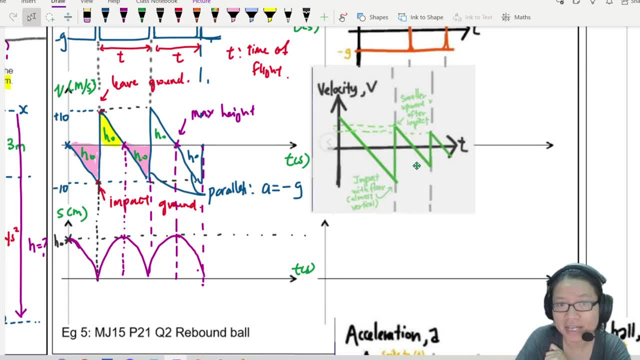 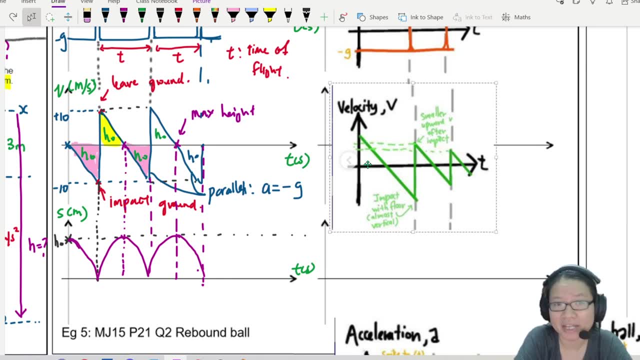 focusing on right now is the characteristic of the graph, namely the characteristic where the peaks and the smaller velocity will get smaller and smaller each time, and then you can see the area gets smaller and smaller each time. so if the area gets smaller and smaller, the rebound height. 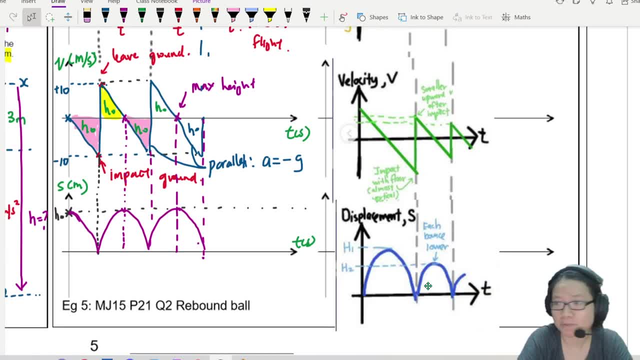 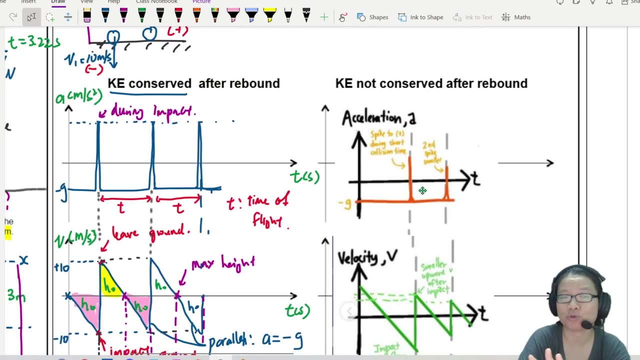 will get smaller and smaller, so you can expect your displacement time graph will look a bit smaller. okay, so the difference between this and this is number one, where we start measuring h, and number two, what the interpretation of the velocity is. so i'm not going to go into that. my challenge to you: 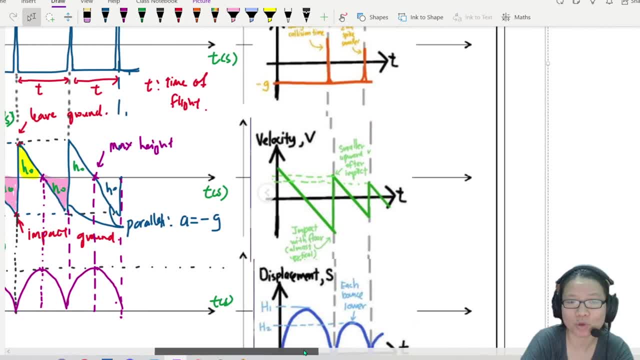 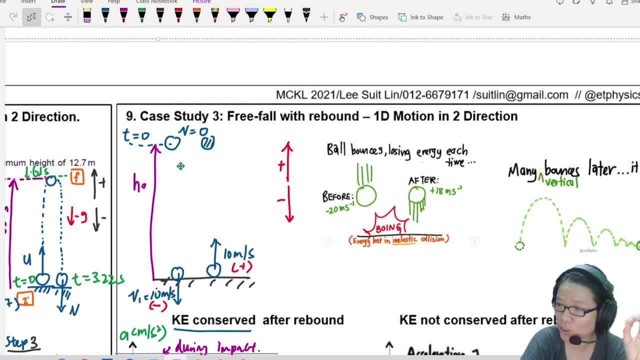 maybe you can draw a scenario for how this one would look like. okay, you could draw a diagram that is similar to mine here. where did we start measuring the h? where did we start measuring the t, and what direction is it considered to be positive? you can draw it here. all right, so this is the 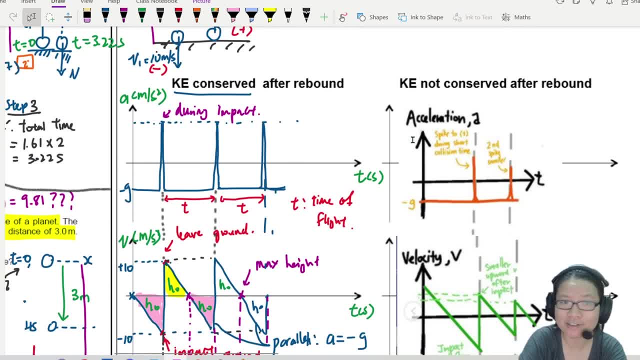 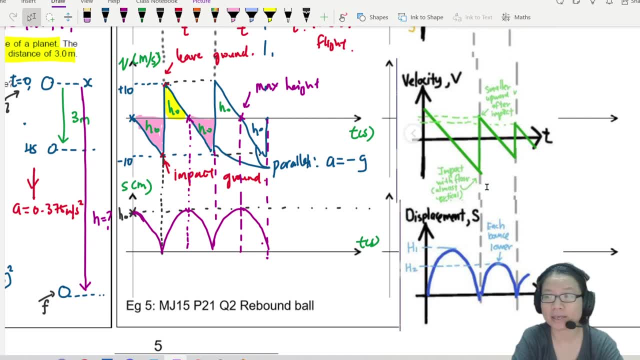 graph. just make sure you know the difference between acceleration- okay, the peaks will decrease- velocity and displacement. you expect to get this graph. so, basically speaking, if you understand the two dimension one, you just combine many, many ones of them together and then you will get the rebound graph, don't worry. okay, if you understand the property, uh, deducing it will be logical, all right. 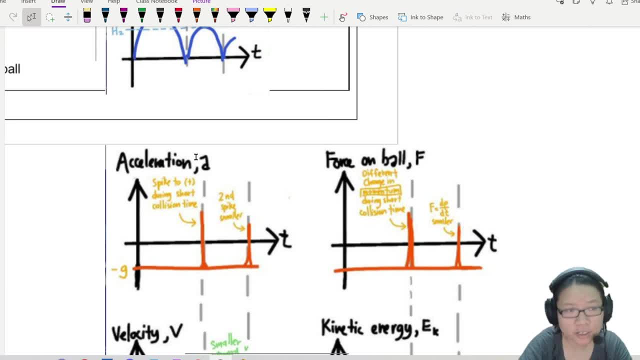 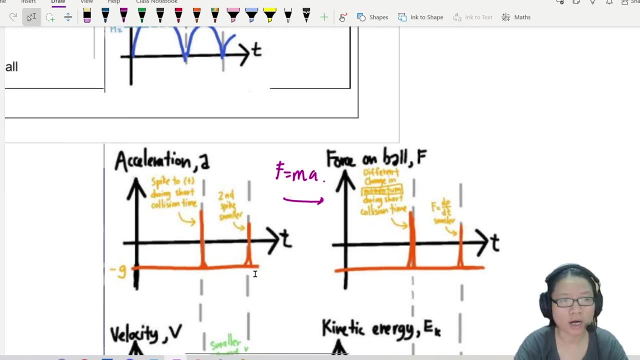 so here's another quick extension for you. based on the acceleration graph, i can actually sketch the force graph. if you don't know this concept, we will level up in the later chapters. but the relationship here is simply because f is equal to m, a. okay, so uh here.